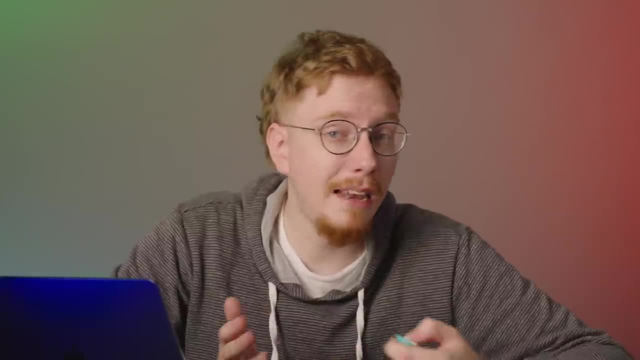 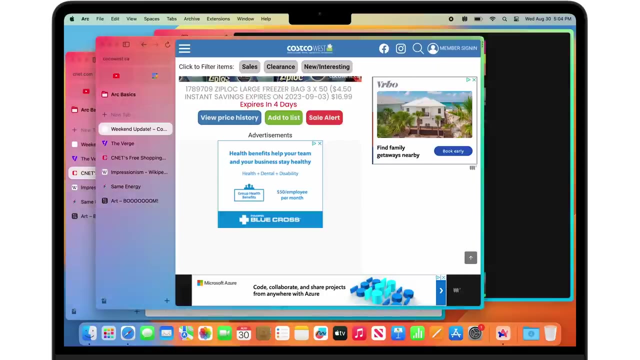 I think it looks beautiful with the vibrant colors, themes and margins. That tab sidebar becomes a liability if you're the type to have multiple small browser windows open at a time. But look what happens when you put it into full-screen mode. 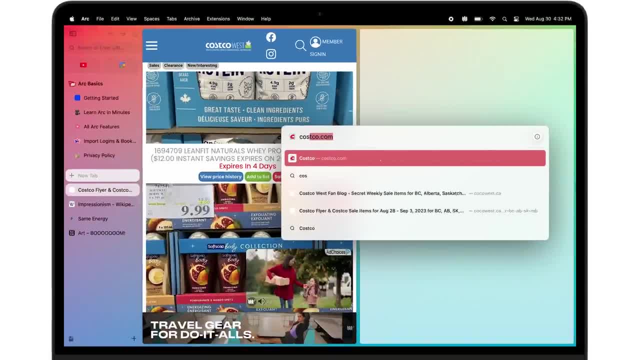 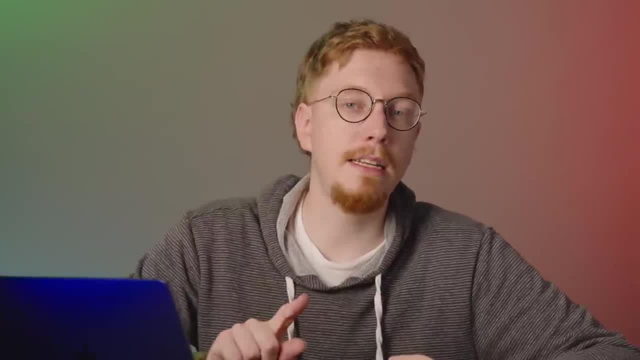 You can take advantage of split-screen to group two or more websites into one tab, just like you can with Mac OS's full-screen mode. Only, this is a little more straightforward and convenient. Plus, a lot of our computer life is spent in a web browser anyway. 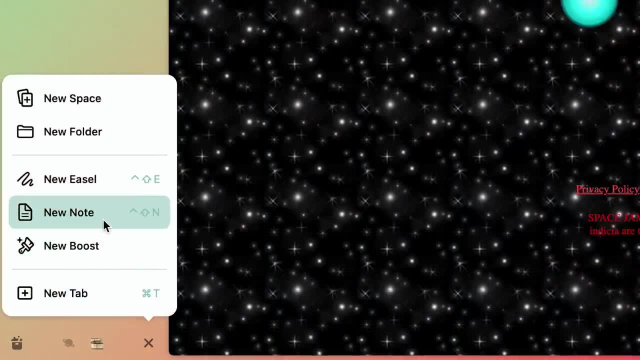 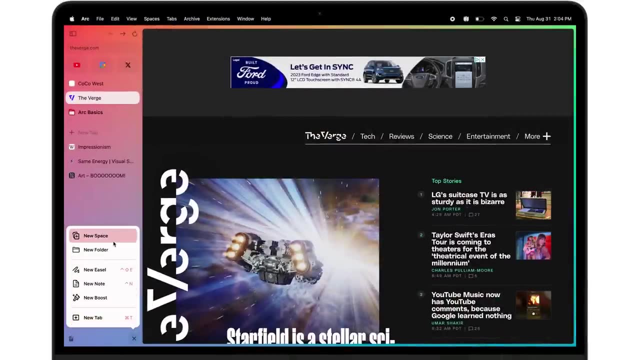 And to keep you there, there's a built-in sketchpad and notepad, which are treated just like any other tabs. What stands out to me is that Arc has a different vision for browsing. You can set up profiles to divide your work and personal life. 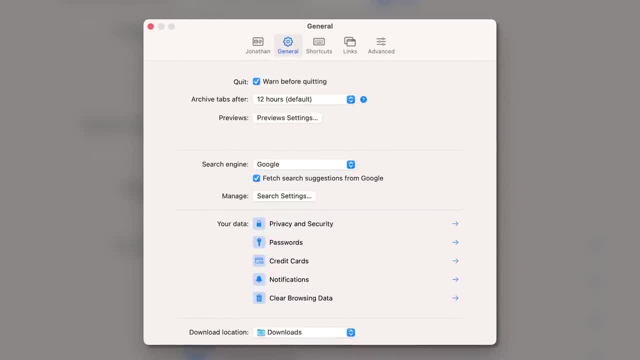 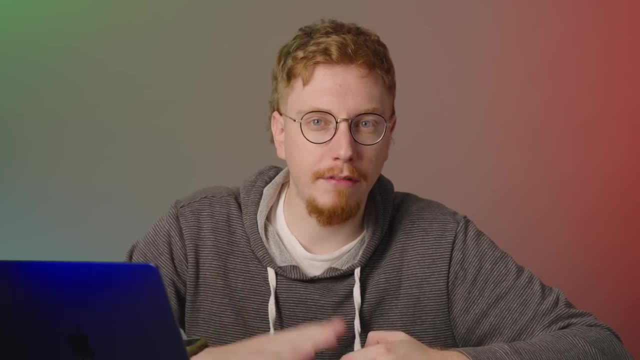 and they're really easy to switch between. But Arc will archive the tabs within profiles after only 12 hours. It's certainly a surprise to open up your computer after a day and find everything you were looking at missing. You have to go into history to get them back or change the setting to 30 days, like I did. 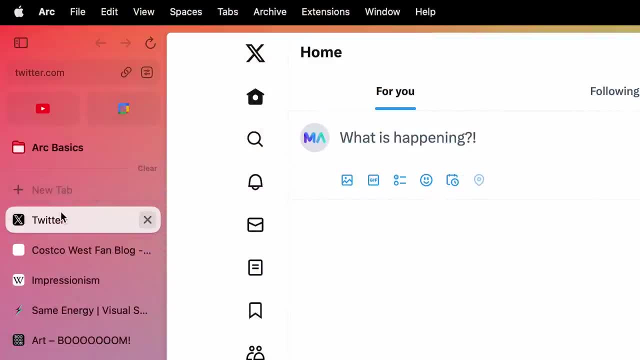 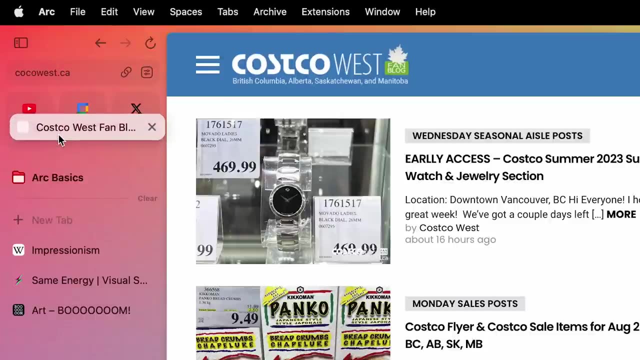 However, there's a well-thought-out process here. Tabs you use all the time across profiles should be favorited as buttons at the top, and tabs you want to keep within profiles should get pinned up here Also. check out this tab layering. 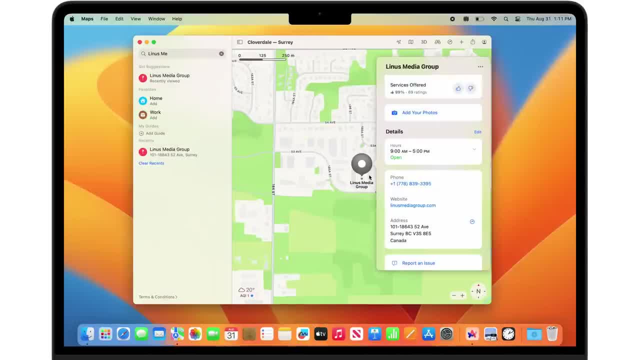 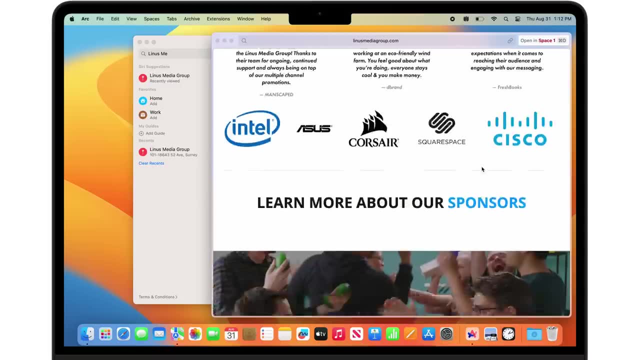 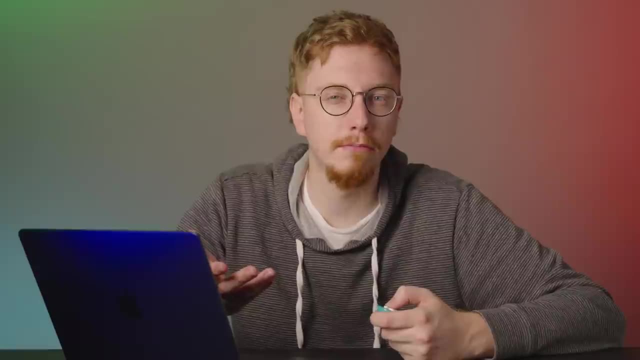 Pretty neat. Outside the main browser window there's mini-Arc windows which appear when you click on a web link from within a Mac app. I like how it helps contain and constrain the web browsing outside of the main browser. If you can adapt to these paradigms, maybe this could help you become more intentional about your browsing. 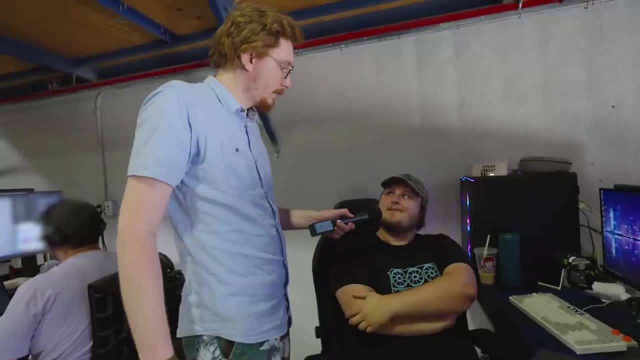 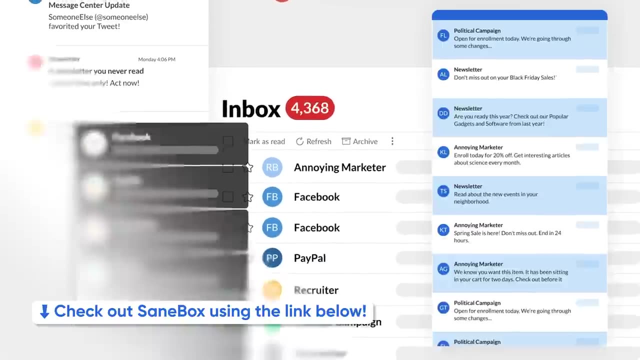 So does it. Well, my colleagues will tell you after a word from this video's sponsor, SaneBox. I don't know about you, but somehow email has become so hard. There's so much to sift through. Well, instead of tediously going through all your emails, 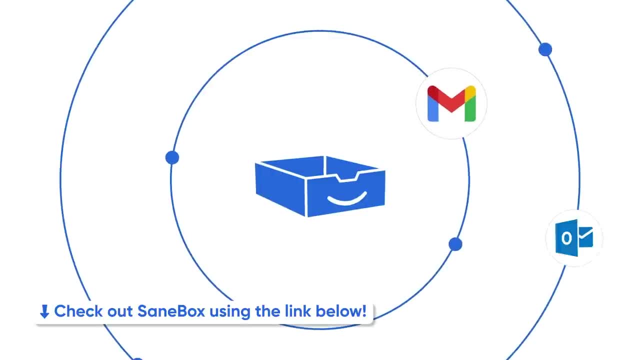 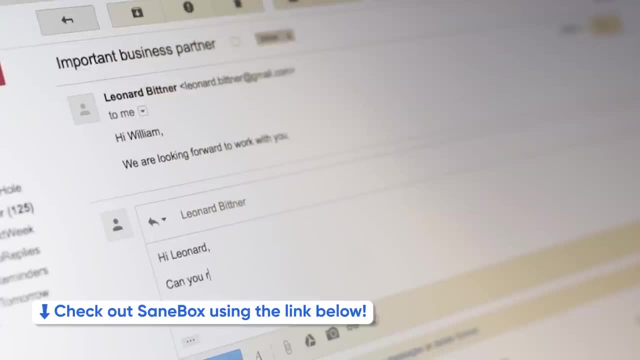 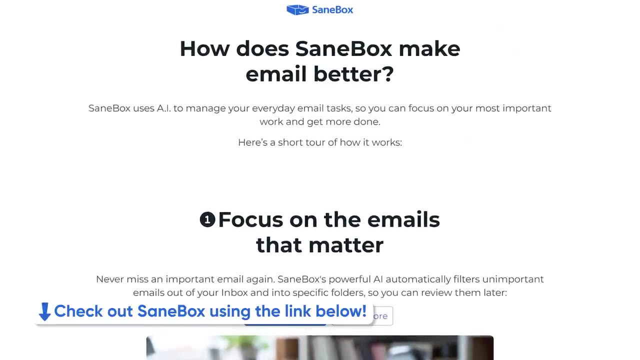 one by one. let SaneBox do the heavy lifting. It integrates with any email client and organizes your incoming mail into appropriate folders, leaving only the important emails at the top of your inbox. Save hours in your week by checking them out at the link below for a free 14-day trial and $25 off a paid subscription. 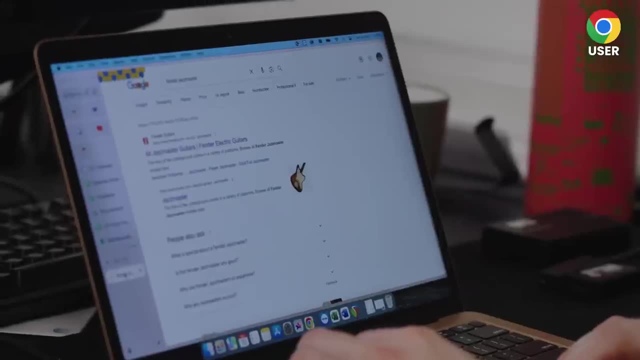 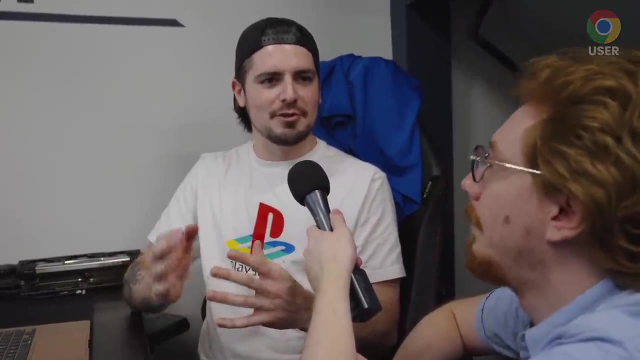 The main goal of it was to sort of clean up all your tabs and have it be a bit more work-focused. I guess you could say You can have a lot more things open at the same time without having a bunch of a bunch of clutter in your taskbar. 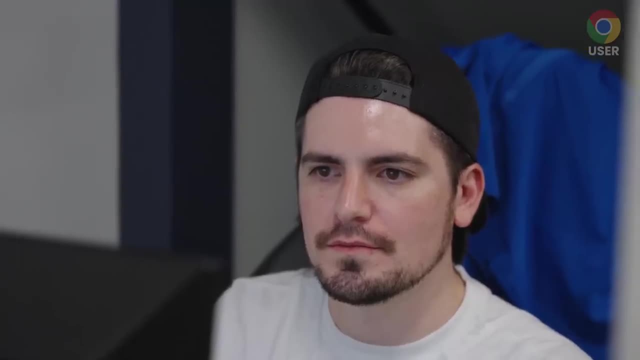 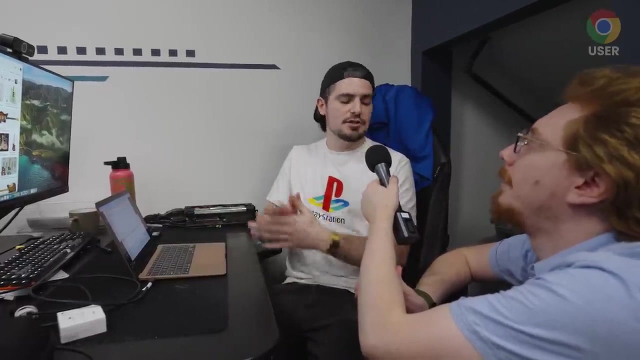 If I'm at work, I sort of have three to five websites that I'm constantly using, so those are just the obvious ones. At home I actually have a different workspace entirely, so I use the space function. So that's just all the stuff that I generally just check either in the morning or after work. 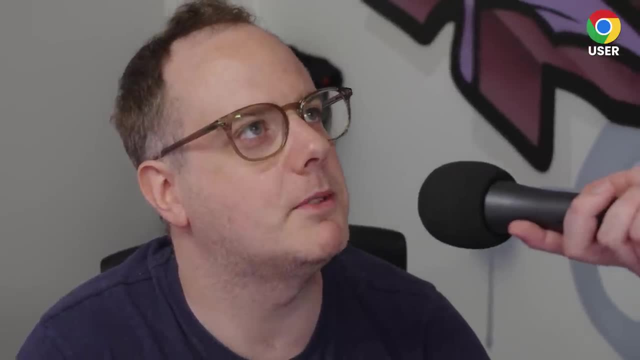 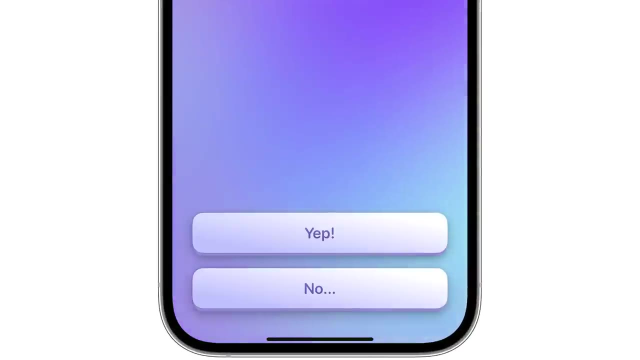 I tried installing it on my phone, but it required a desktop to install for some reason. The phone version of Arc is interesting. I like its design a lot because buttons feel like buttons, But it is hard. It's not a working document. 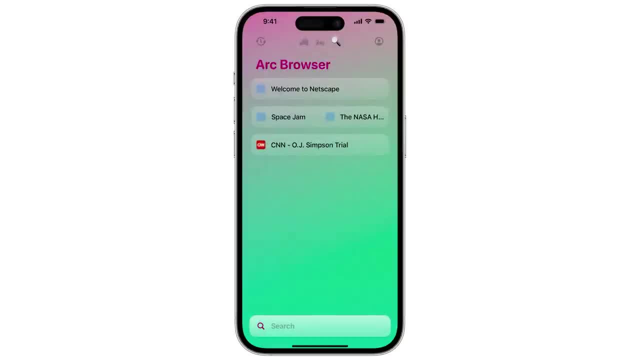 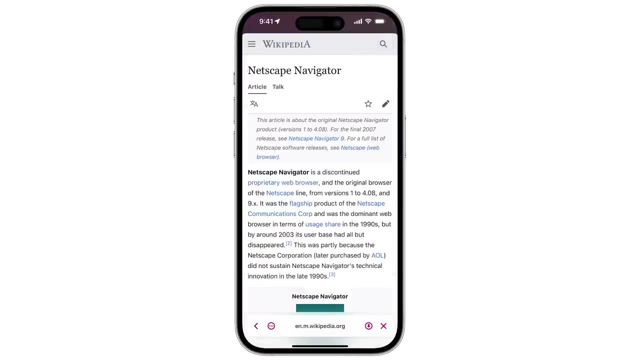 It feels like it's actually stuck in a background and probably not going to work. If you're a desktop user, this kind of thing really needs your attention. I'm going to show a few things about Arc One. it's fully unfinished. 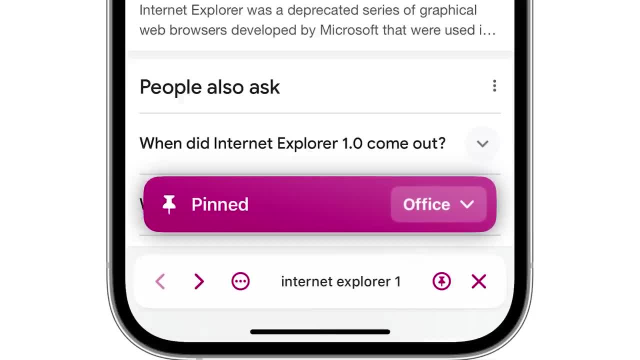 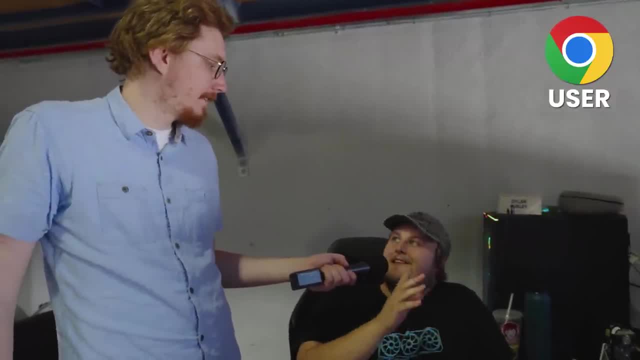 It syncs to your desktop surfing sessions via iCloud, letting you carry on from what you were looking at there. However, you cannot contribute to it by adding a new tab. Instead, you can only search in one temporary tab that's gone as soon as you swipe it down. 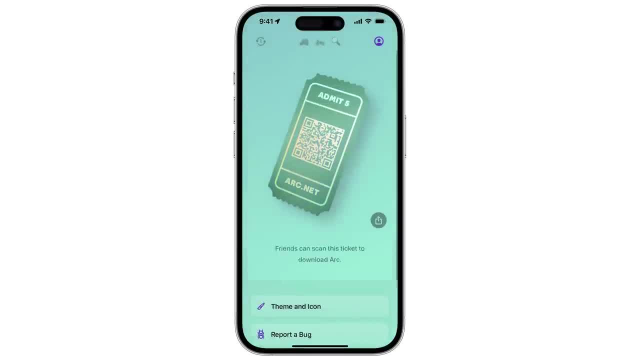 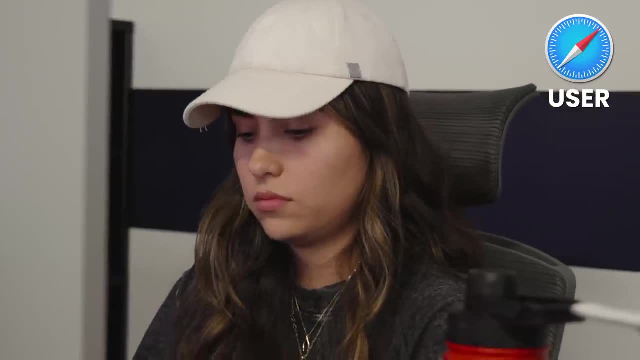 Unless you pin it. I prefer it on mobile over desktop. It has cute little animations. At first I like it. I really like the UI. I think it's pretty pretty and design-wise I like it. But then, when I used it, I didn't like it as much. 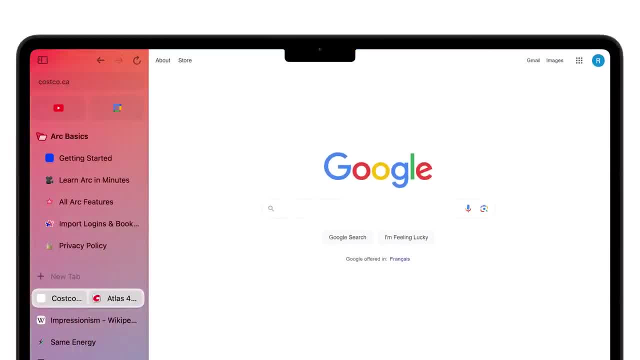 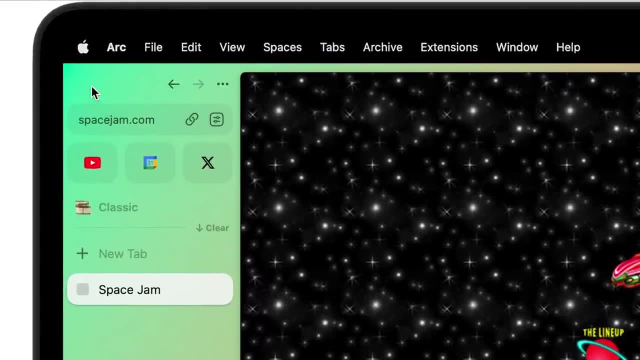 because it's just like Google Chrome, but more beautiful. I have my own minor gripes too. The back button and address bar are too small and insignificant relative to their importance to surfing, But these are small things that wouldn't prevent me from switching. Would you switch to Arc? I don't think so, But you would still stick with Safari. Yes, Wow, I'll try it out. I'm open to anything that will make my life better. Yeah, as of now, I have fully switched to Arc. 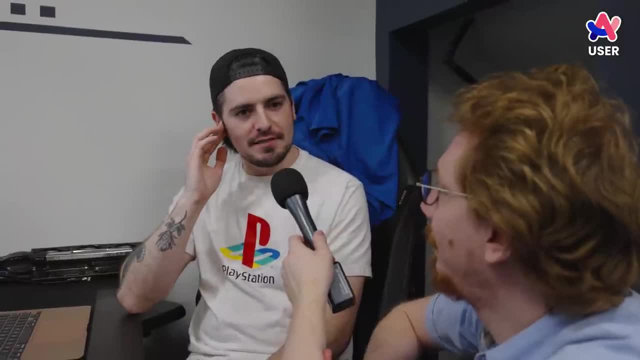 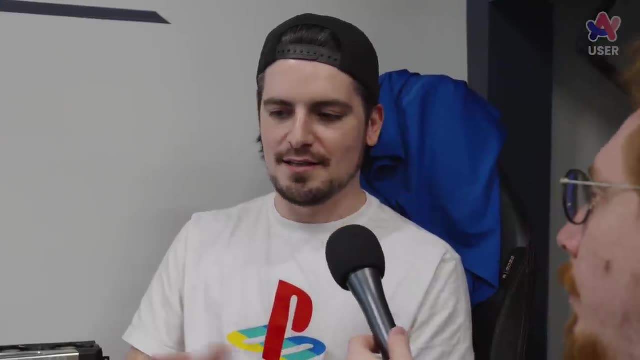 Yeah, Whoa, that's crazy. Yeah, it was really easy with all the importing that it allows from Chrome. It just brings everything over. You just had to make an account, sync everything up and it worked. What? Hold on a minute? 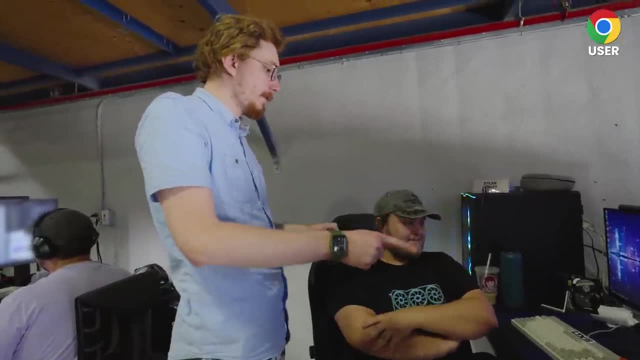 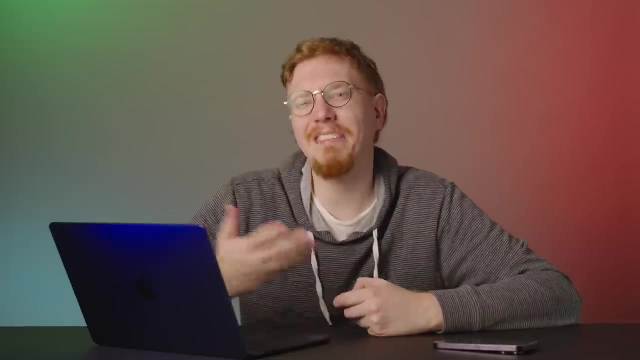 I wouldn't mind it on the PC, It'd be kind of useful. So if Arc was available on the PC, then would you switch? Yeah, The streamlined design like a Mac but on the PC would be great. I'm still quite indifferent to switching browsers. 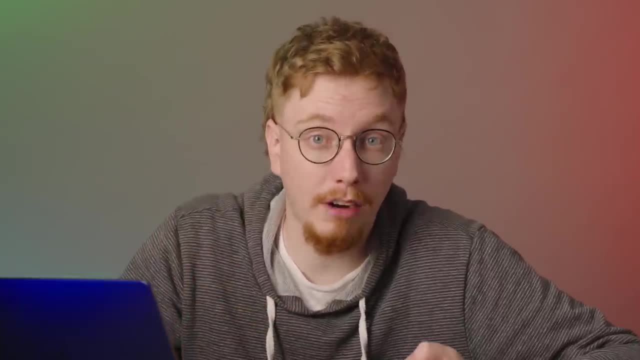 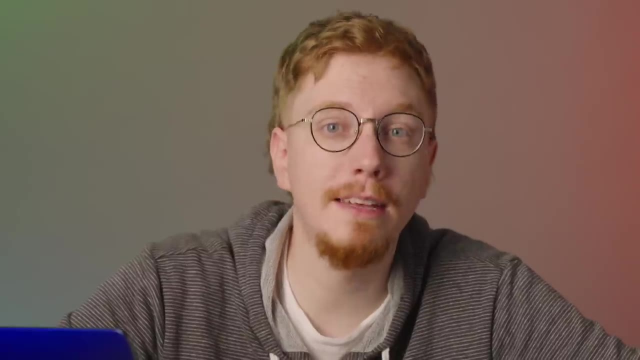 I go where the wind takes me. I started using Safari full time because I cover Apple and that's the browser. Apple made some big updates to Safari last year with tab groups and their own take on profiles, But because Apple's stuck in their flat design ways. 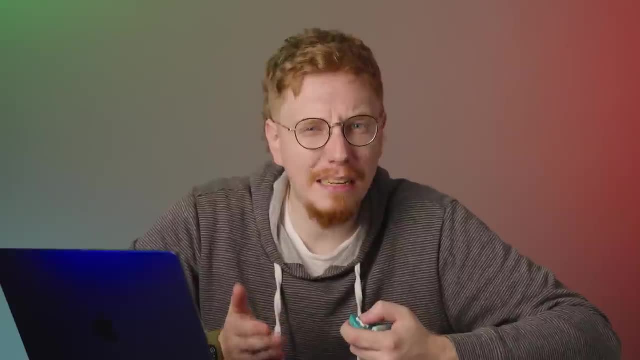 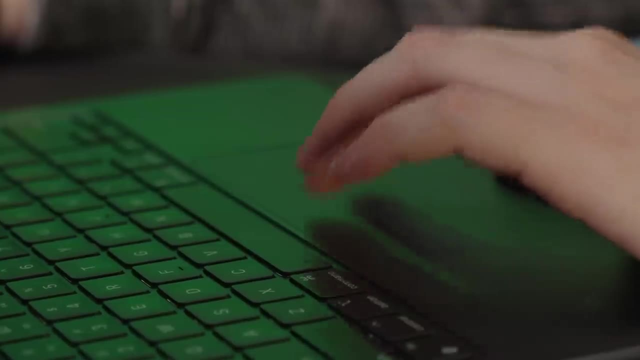 and they built these features in a well-established interface. I found it difficult to incorporate them into my surfing habits. I'm glad I'm giving Arc a try thanks to this video, But does this mean I'm committing to an Arc era? I think I might just do it. 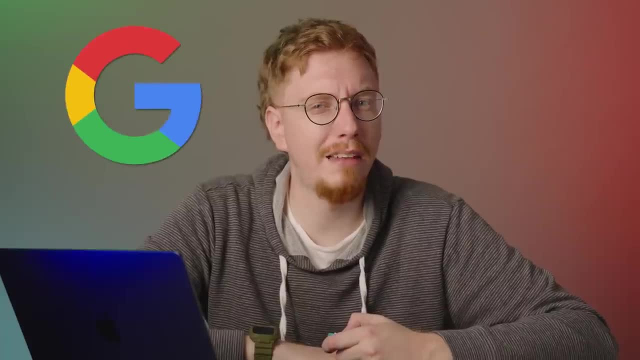 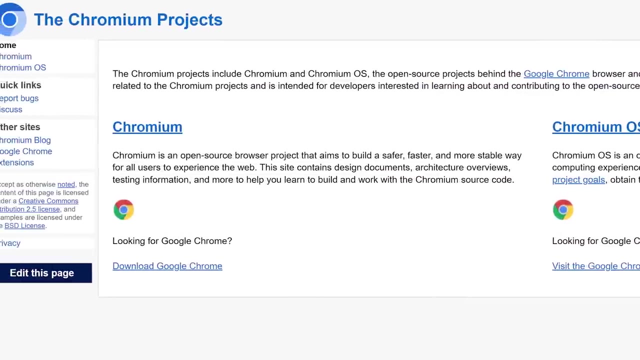 But there are two niggling problems: Google and the money. Arc is built on Chromium, the free, open-source version of Google Chrome, available for developers to build their own browser on top of That means they all have the same engine and have all the same base features available. 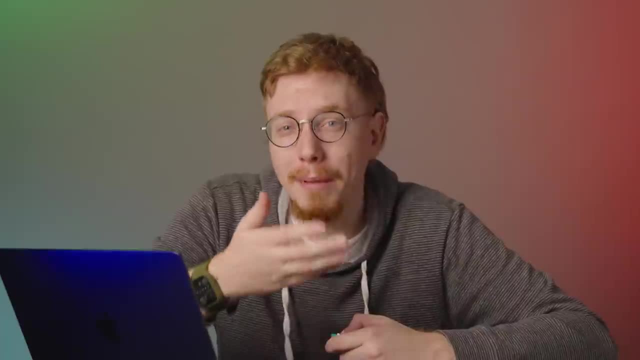 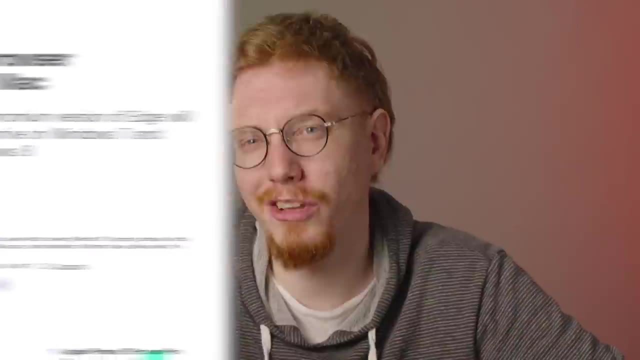 making it easy for chromers to switch over. Even Microsoft, who dominated the browser space 20 years ago with Internet Explorer, has switched to their Chromium-based edge. Yet it means that Google dominates in yet another layer of the web space, and I'm a little tired of it. Chromium may be open-sourced, but Google still has control over it. So even if you're not using Chrome, the web is still being optimized for it in other parts of Google's business. Like most other browsers, Arc is free. Free with Google means monetized with their advertising. 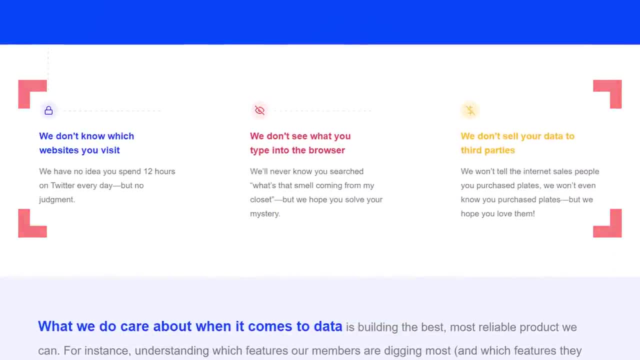 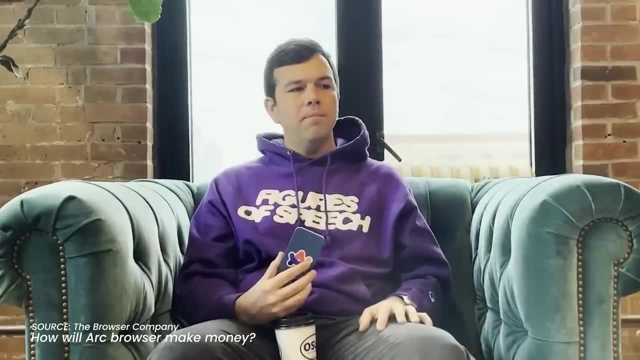 and surveillance, But Arc makes a big deal about not monetizing your data, So they're still going to be looking for ways to earn money differently. One way to monetization is Arc for Teams and saying, hey, if you're working at a company. 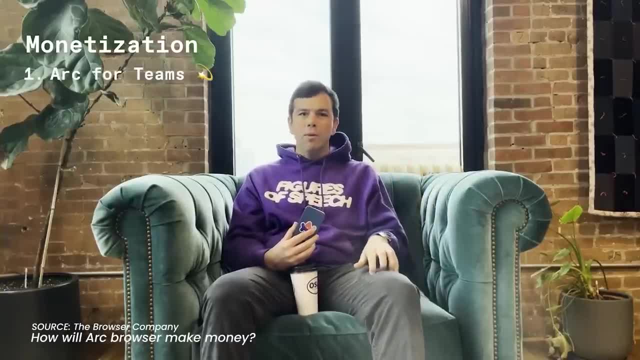 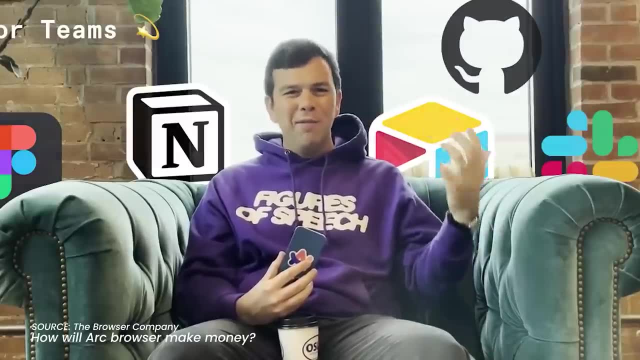 how do we make it so? the best way to work together is in Arc with Arc together, Kind of the way that Figma, Notion, Airtable, all these companies monetize. I mean it's really great You give it away to individuals for free forever. 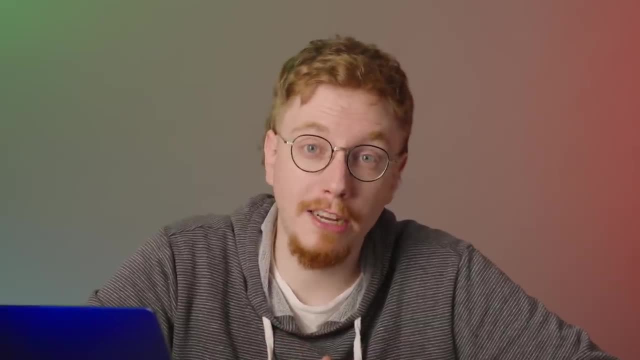 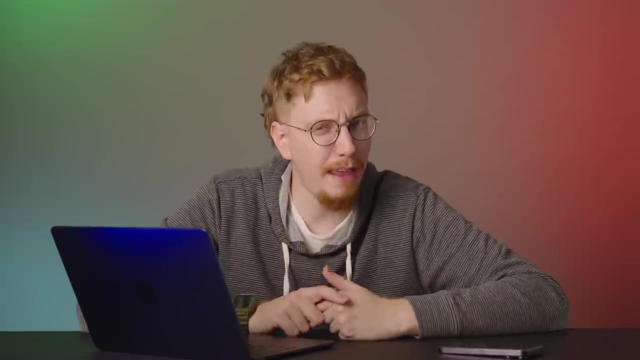 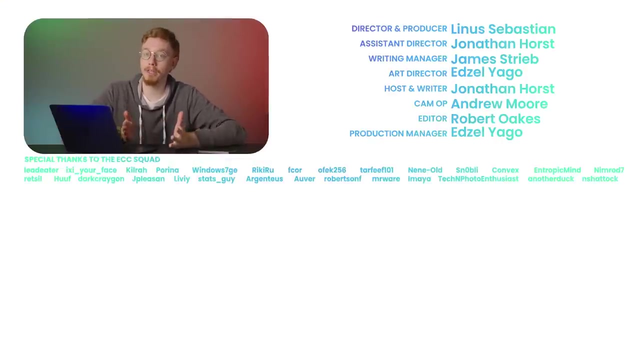 and then you charge their companies. Exploring monetization strategies that break from the convention of us users being the product is laudable, But would you or I pay for Arc? Depends on the price. Thanks for browsing through this MAC address. If you surf the web, give this video a like. 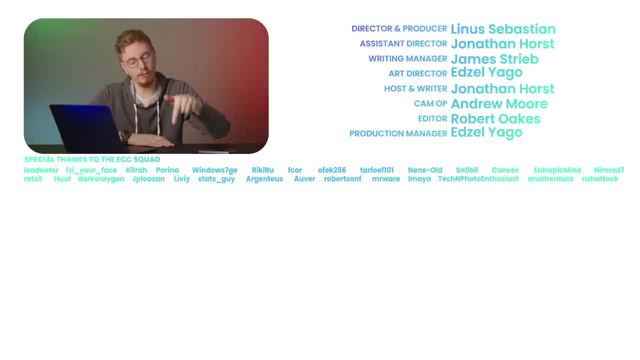 And if you surf the waves well then you might as well subscribe. I'm curious, in the comments below, what browser you currently use and what errors you've had in the past, And would you try Arc?